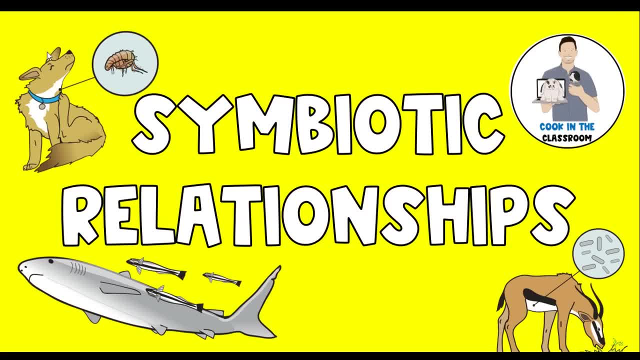 Today I'm going to teach you all about symbiotic relationships, everything that you need to know to be able to identify which type of symbiosis people are talking about, because you're going to encounter practice problems and questions where you have to identify the specific type. 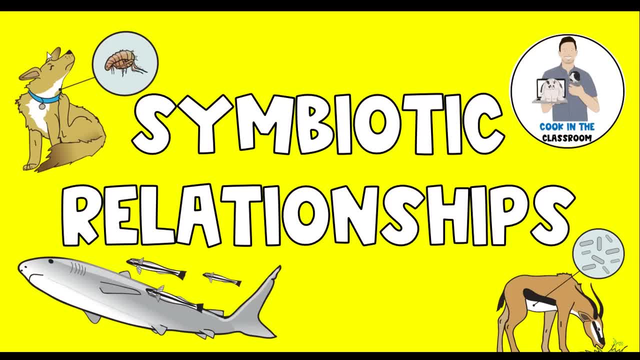 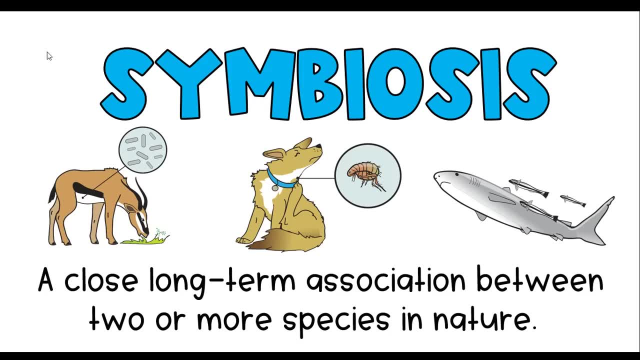 of symbiotic relationship. But before I do that, I want to tell you what is symbiosis itself. What does that mean? Symbiosis is a close, long-term association between two or more species in nature. So what that means is these animals interact in nature and in the wild, and they have for a long 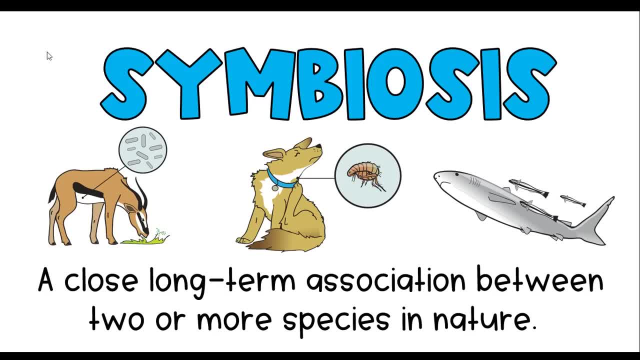 time. So these are not just two specific animals interacting, but the entire species interacts in nature And those interactions are really important And we're going to talk about the different types of symbiosis. So what does that mean? Symbiosis is a close, long-term association. 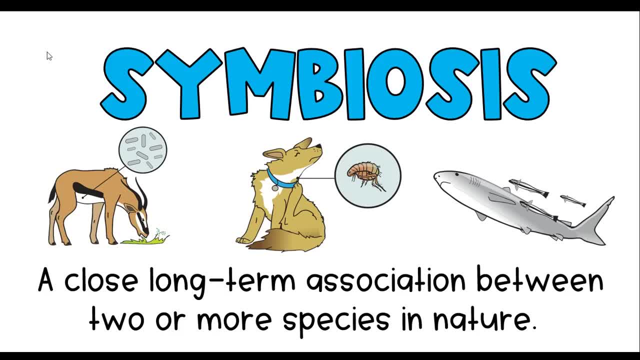 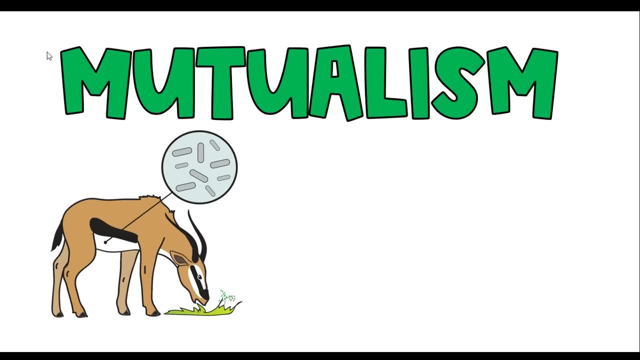 ways that they can affect both species in that symbiotic relationship. The first way is mutualism. Mutualism is a symbiotic relationship in which both organisms benefit, And when we say benefit we mean something good happens as a result of this relationship. So 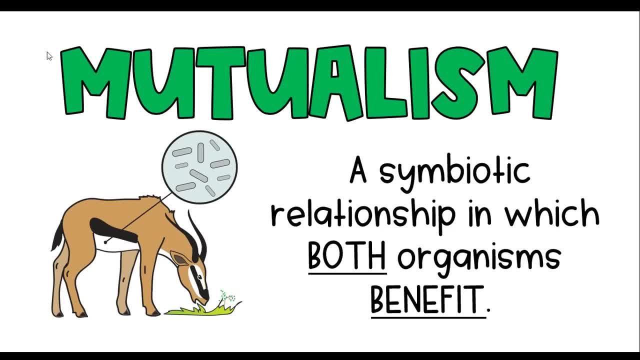 this is a good thing for both organisms. In the example we have what I believe is a gazelle or an ibock, I'm not sure, but the bacteria is what you see in the circle And this is a symbiotic relationship that is mutualistic. The bacteria which we might think of as a bad thing, that might. 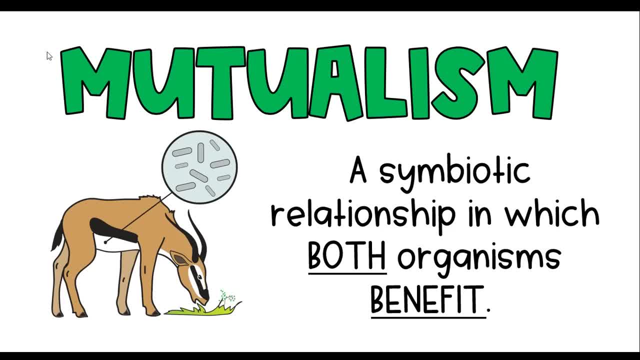 get us sick. they actually live in the intestines of this animal and even us as humans, And they help us digest food that we can't break down on our own. And when they digest that food, it releases certain vitamins and nutrients that help us as humans and this animal- The animal- is getting 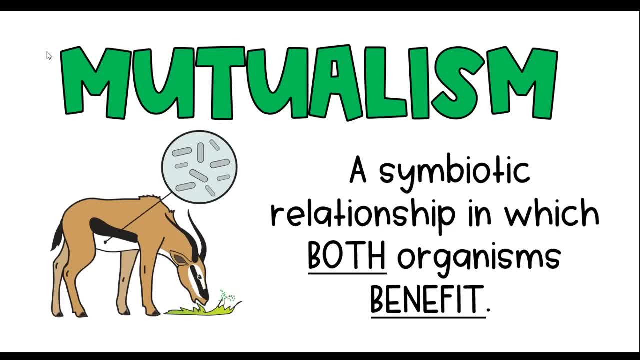 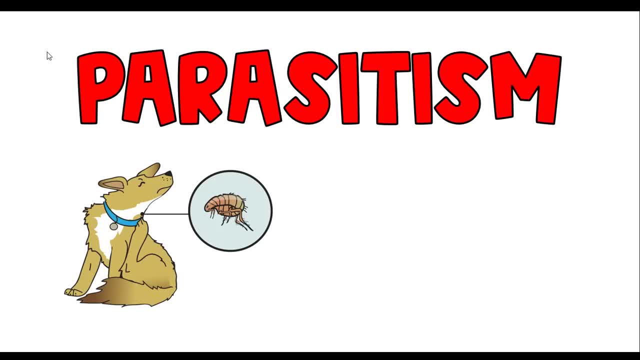 that digestion, but the bacteria are getting food out of it, So they both get something good out of it, And that is what mutualism is. The second type of symbiotic relationship is parasitism. Parasitism is when one organism benefits and one is harmed. So when one is harmed, that means it's 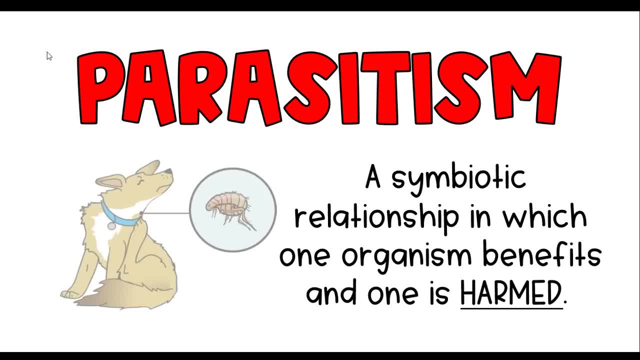 not good, And that means that one organism is not good And that means it's not good And that means for the organism that's harmed. and you can see this example of the dog and the tick. the tick is latching on to its host and the host is the organism that is having things taken from it. 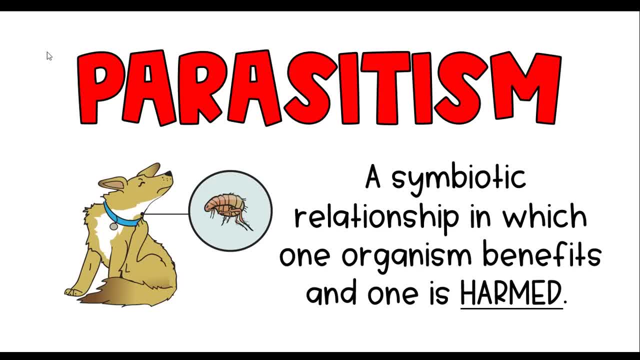 the tick will take blood from the host and that means the dog is losing nutrients, losing blood, and in addition to that it can also get diseases, which is definitely not good for the dog. so it is harmed. but the tick is getting food and a host to live off of, which means it's benefiting. 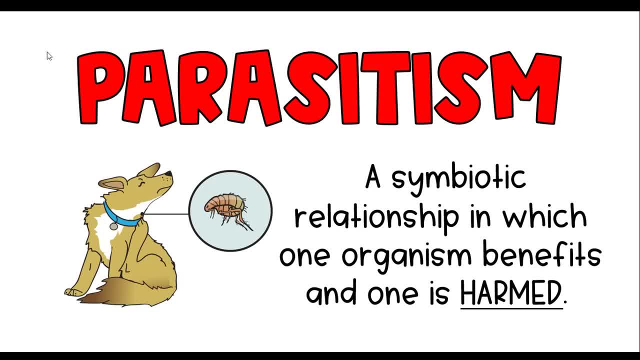 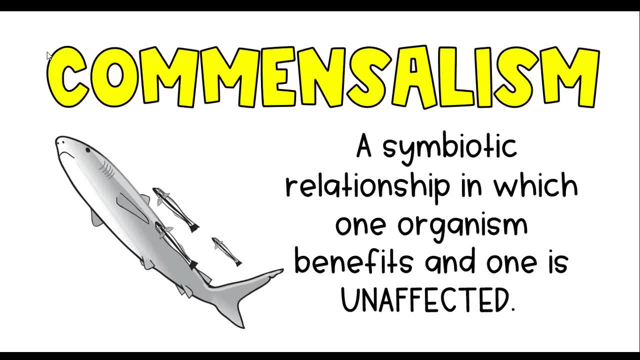 so one benefits and one harmed is parasitism. the mensalism is when one organism benefits and the other is unaffected. when we say unaffected, we mean that one organism doesn't really care either way. it's not positive, it's not negative, it just doesn't matter to them. 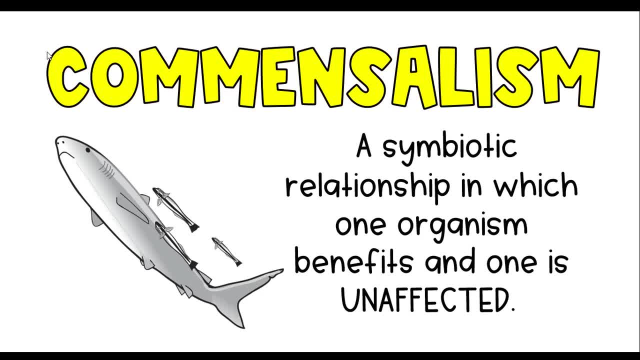 so unaffected, and in this example we have the shark and the remora fish. the shark swims along, eats and, as it's eating, these little remora fish swim right beside it. now, the first thing my students always ask me is: don't the remora fish get eaten by the shark? and the answer is no, they're. 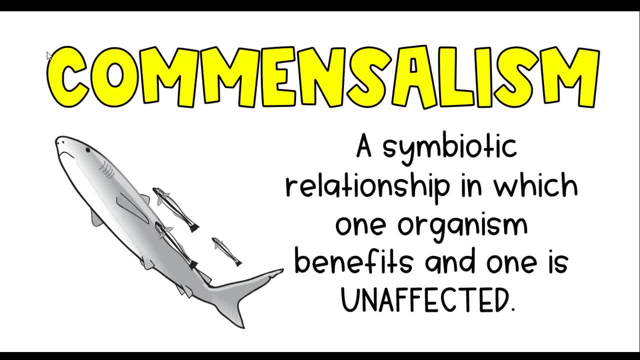 not prey of the shark, so they swim alongside it. the shark eats and as it eats, food falls out of its mouth. if you've ever seen a shark, it's not prey of the shark. it's not prey of the shark on national geographic. there's just food flying everywhere and that's the food that the remora fish. 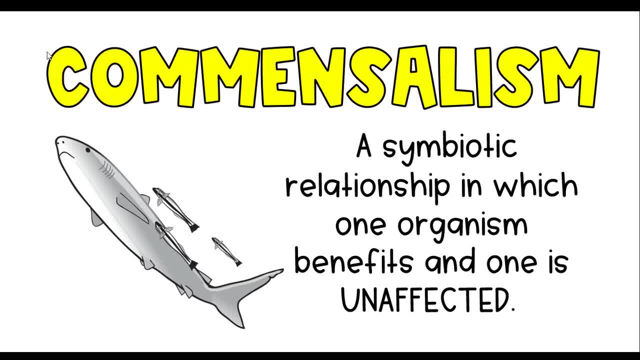 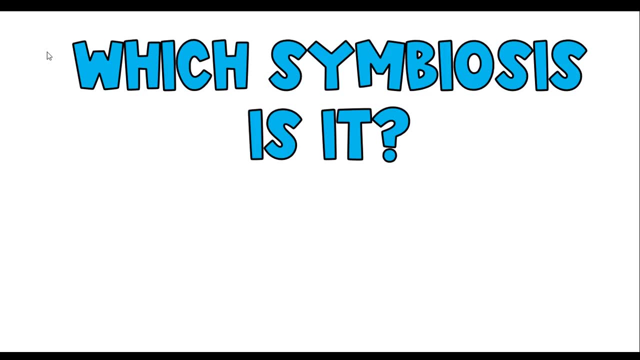 gets, because it was just going to go to the ocean floor, so the shark does not care. but the remora fish is getting protection because they're swimming by the big bad shark and they're also getting food, all right. so it's really important that you're able to go through these questions. 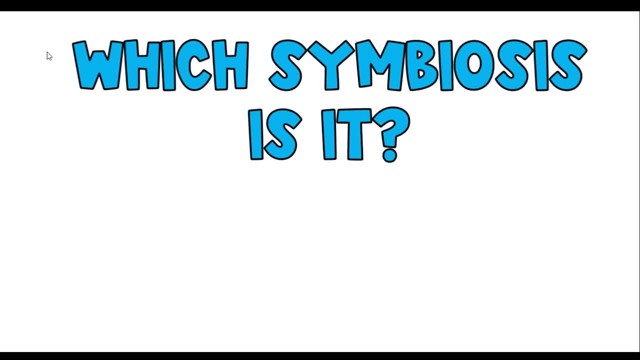 and types of practice problems and identify which symbiosis is it. so i'm going to give you some examples and what i'd like you to do is read along and think along which type of symbiotic relationship is describing, and then you see, if you're right, as i tell you the correct answer. all right, in this one we have the rhino, which you can. 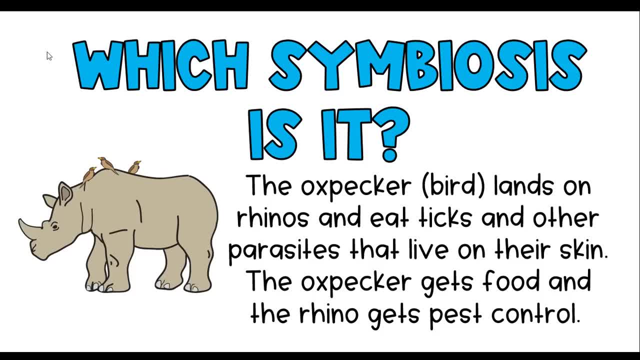 see, and the ox pecker. the ox pecker, the bird, lands on rhinos and eats ticks and other parasites that live on their skin. the ox pecker gets food and the rhino gets pest control. now the first thing that you want to do in any symbiosis question is ask yourself: is it good or bad for each animal? so let's say: 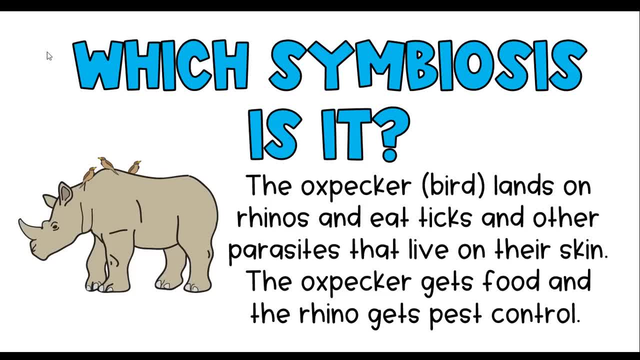 the ox pecker. it says that they get food and i like food. most animals like food, so that's a good thing. now the rhino gets pest control, which means that the ticks and other parasites are eaten by the bird, and we know that parasites take from the host, so we don't want parasites on us. so the rhino is. 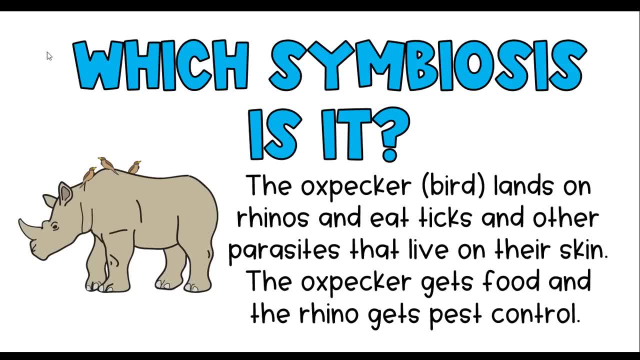 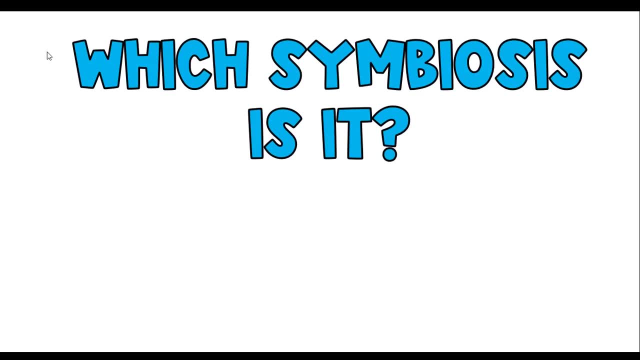 also getting something good out of this, which is pest control. so, if they both benefit, which type of symbiosis is it? well, if you answered mutualism, then you are correct, because both benefit in this example. all right, the next example which symbiosis is? it is the orchid and the 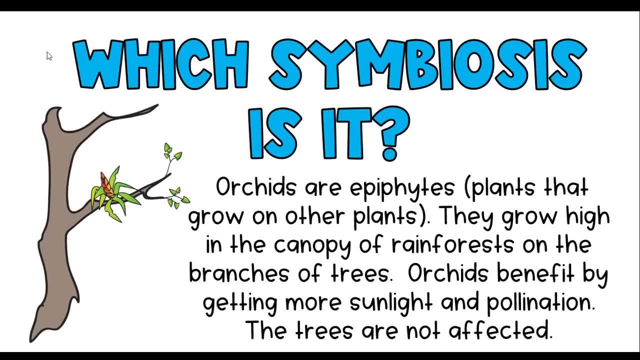 tree, the orchid, which is an epiphyte- i'm hoping i'm saying that correctly- it's a plant that grows on other plants or trees. they grow high in the canopy of rainforest, on the branches of trees which you can see to the left. orchids benefit by getting more sunlight and pollination, and the 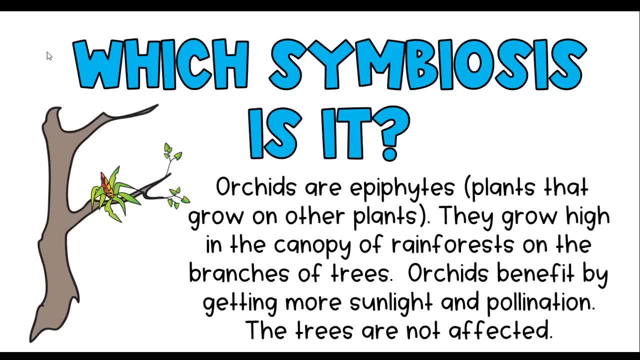 trees are not affected. so in this question again we're going to ask ourselves what happens to each one. the orchid, it says, benefits by getting sunlight and pollination and the trees are not affected by getting sunlight and pollination and the tree is unaffected. so if one is benefited, 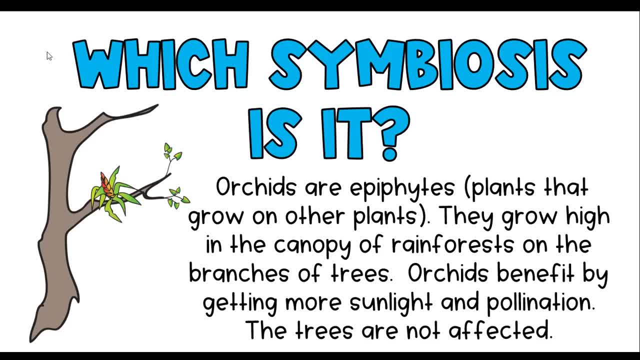 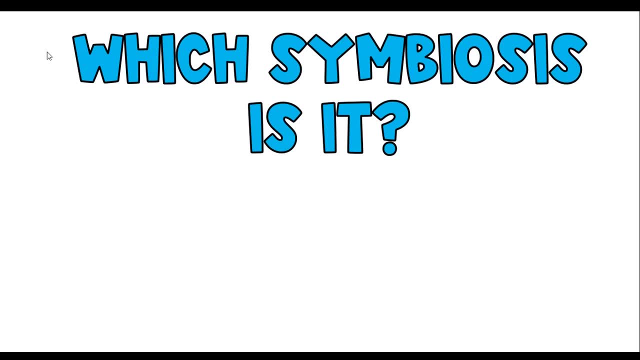 and one is unaffected. which symbiosis is it? if you answered commensalism, you are correct, because we know that when one benefits and one is unaffected, that that is the type of symbiotic relationship. all right, the last, which symbiosis is it? we've got the brown-headed cowbird, which? 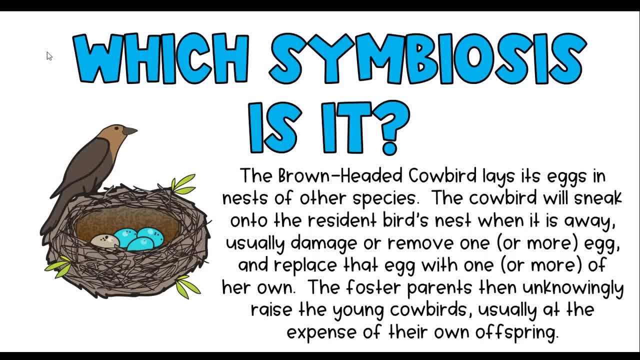 lays its eggs in the tree and the tree is unaffected. so if one is benefited and one is unaffected in the nest of other species, the cowbird will sneak in the nest of other species. the cowbird will sneak into the resident's bird's nest when it's away, usually damage or remove one or more egg and 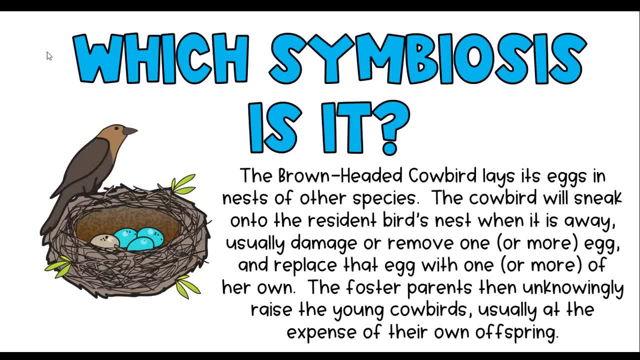 onto the resident's bird's nest when it's away, usually damage or remove one or more egg and replace that egg with one or more of her owniet. in the nest of another bird and replace that egg with one or more of her own, meaning she's laying her egg in the nest of. 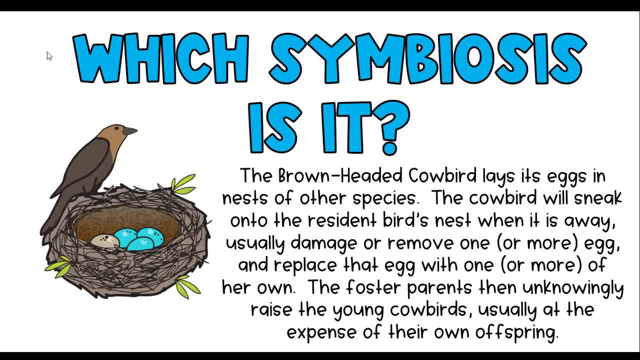 another bird and kicking some of the other bird's babies out of the nest. the foster parent then another bird and kicking some of the other bird's babies out of the nest. the foster parent then unknowingly raises the young cowbirds, and usually at the expense of their own offspring, isaac. 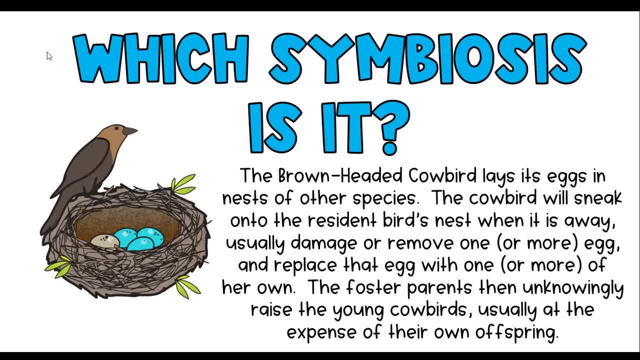 DANIELS two's orange brown hunts and purple cricket bergen the hind cat, green isaac, which means that this is good for the cowbird but it seems really bad for the other host parent. So if we have one that benefits and one that is harmed, 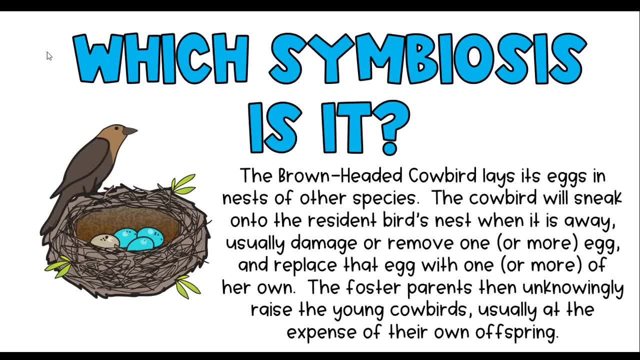 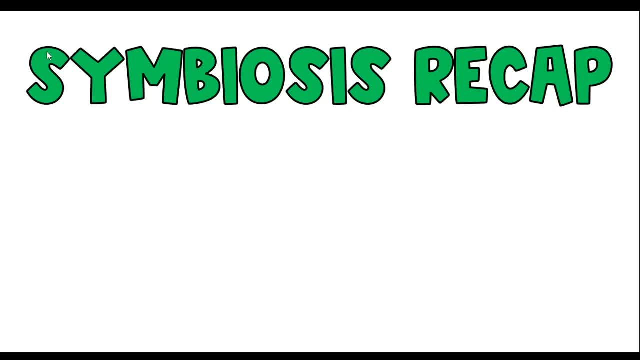 which symbiosis is it? If you answered parasitism, you are indeed correct. One benefits and one is harmed. All right, I'm going to give you a symbiosis recap. I do want to say, if you want more practice, problems. 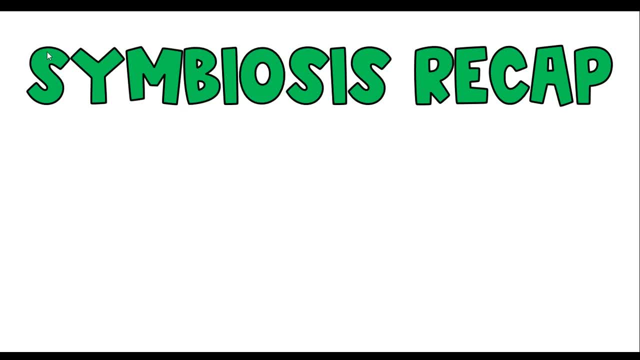 if you're a teacher out there and you would like to give your students some practice problems, you can head to the link in this video and you can go to my Teachers Pay Teacher store where I have symbiotic relationships, practice problems, and it's automatically going to grade itself. 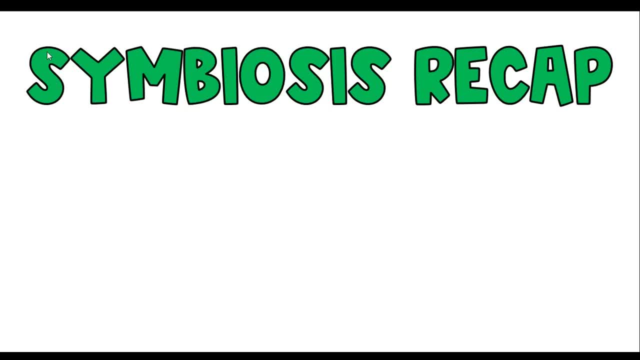 in something you can post in Google, Classroom or wherever you post things. But symbiosis has mutualism where we both benefit and we know symbiosis is a close, long-term association between two species in nature. Parasitism is when one is benefiting in the relationship. 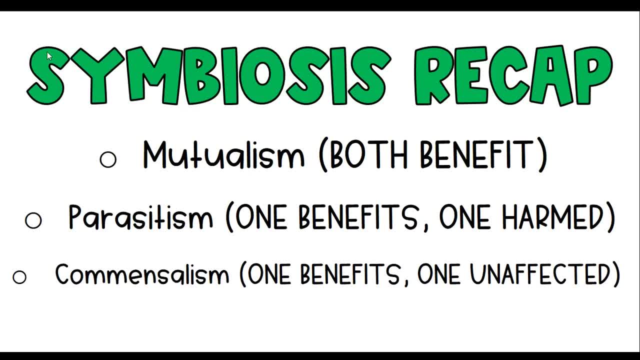 and one is harmed, And commensalism is when one benefits and one is unaffected. One other term that often comes up in this topic is coevolution, which is when two organisms evolve together and change over time, But I'm not really talking about that too much in this practice problems. 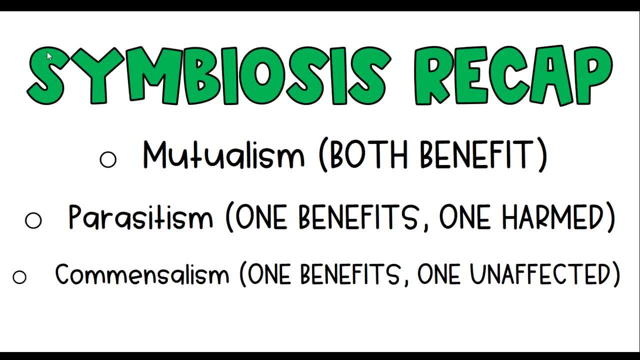 but that is one important thing to also note. So if you have any questions, if you have any questions left for me, feel free to ask down below in the comments of this video and I will answer them for you. And don't forget to like and subscribe. 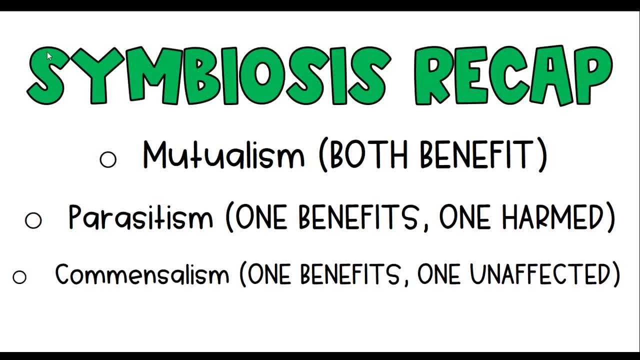 And I hope that this video has taught you about symbiosis and symbiotic relationships. And until next time, happy teaching and I'll see you in the classroom.